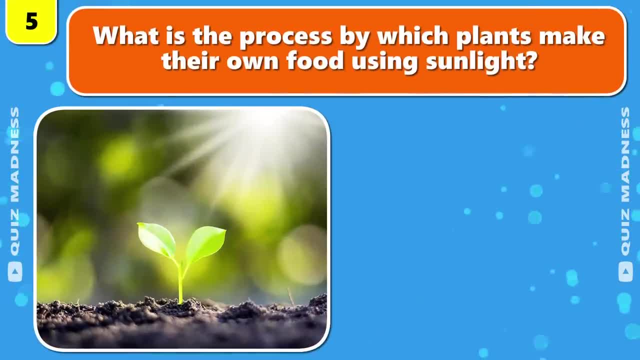 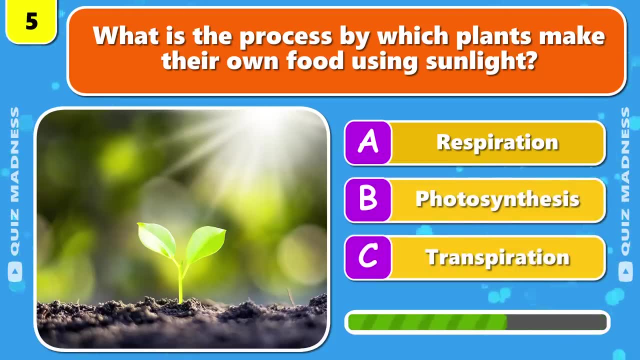 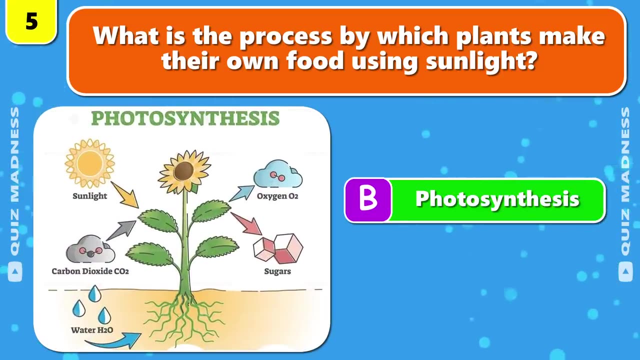 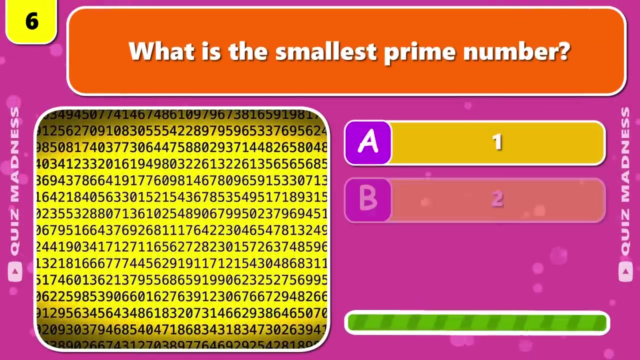 Question 5.. What is the process by which plants make their own food using sunlight? A Respiration, B Photosynthesis or C- Transpiration? The answer is B- Photosynthesis. Question 6.. What is the smallest prime number? Is it A, 1, B, 2 or C 3? 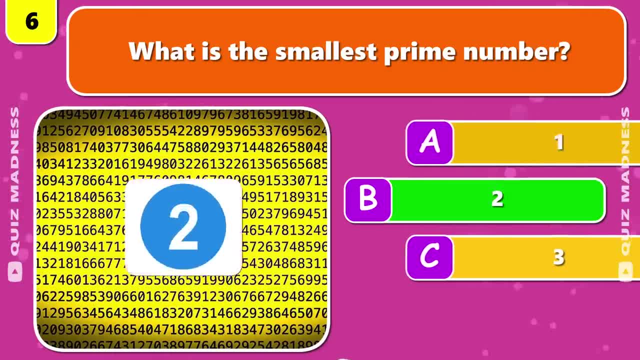 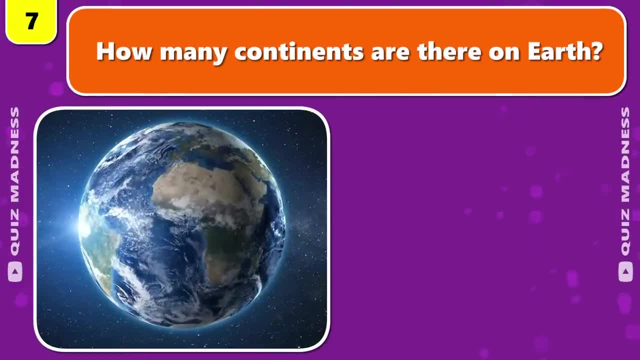 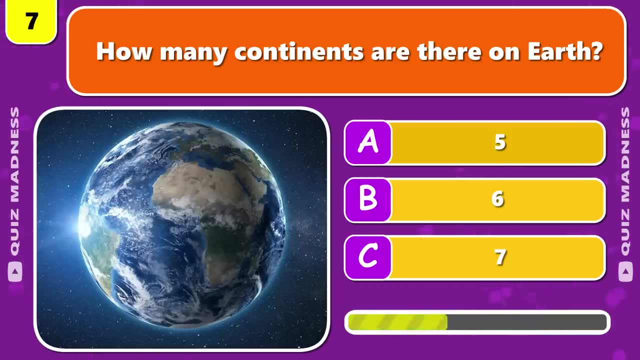 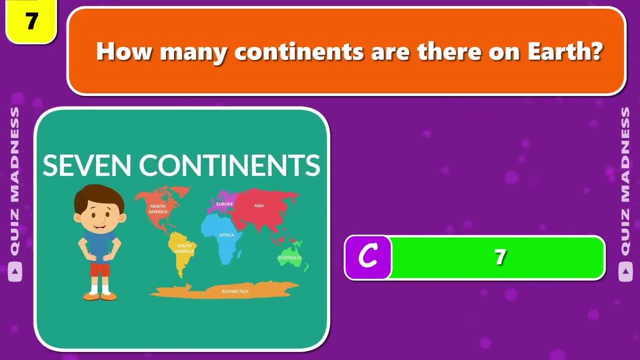 It is B 2 Question 7.. How many continents are there on Earth? A, 5, B, 6 or C 7? Correct, The answer is C 7, Question 8.. What is the largest ocean on Earth? 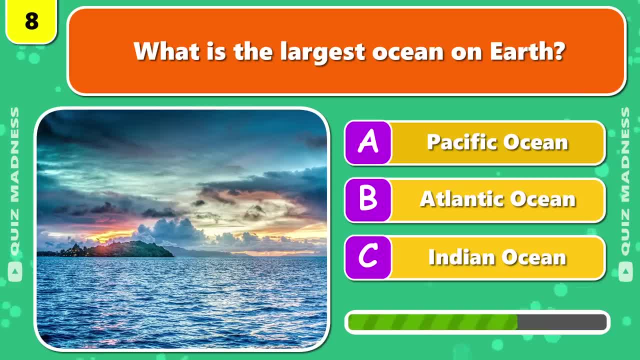 A- The Great Black Sea, B Space Or C space. Question 9.. What is the largest ocean on Earth? A- The Great Black Sea, B Space. Question 10.. What is the largest ocean on Earth? Pacific Ocean. B- Atlantic Ocean. 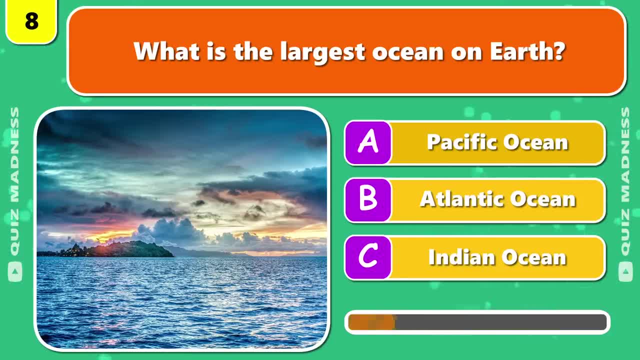 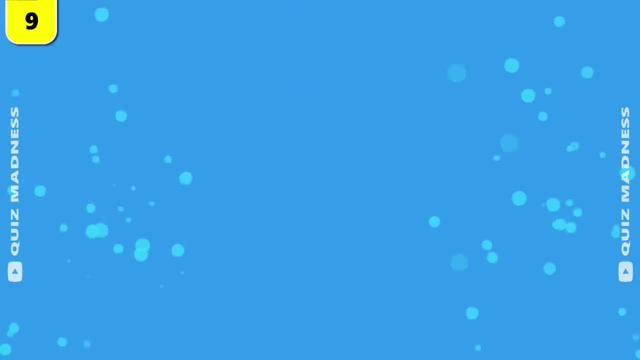 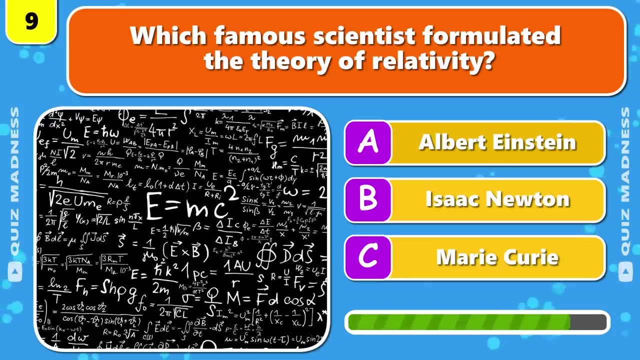 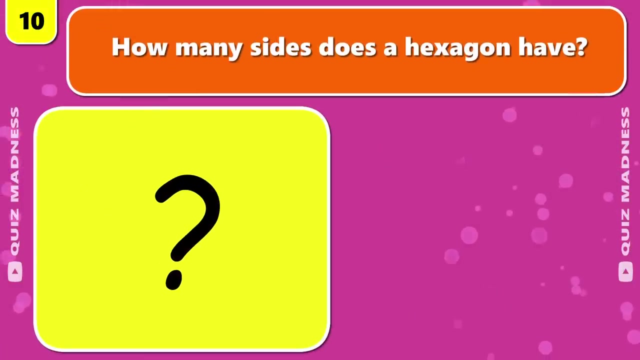 or C- Indian Ocean? Correct answer is A- Pacific Ocean. Question 9.. Which famous scientist formulated the Theory of Relativity? A Albert Einstein, B- Isaac Newton or C- Marie Curie? The answer is A- Albert Einstein. Question 10.: How many sides does a hexagon have? 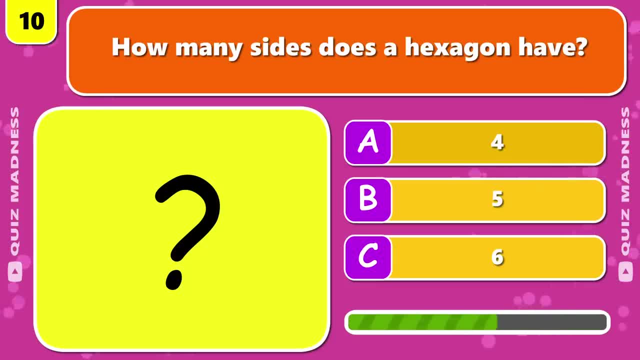 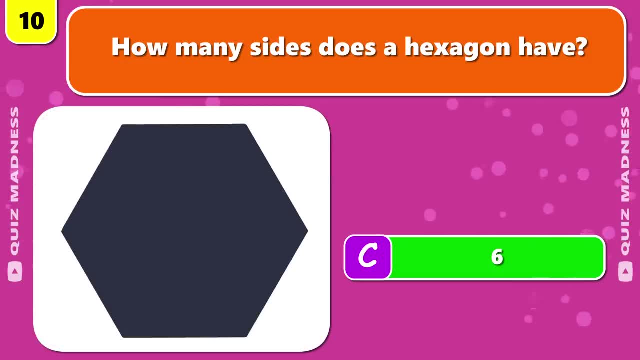 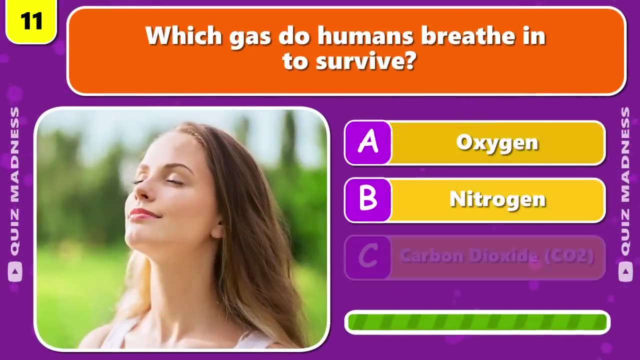 Is it A Four, B Five or C Six? Yeah, a hexagon has C, Six sides. Question 11.. Which gas do humans breathe in to survive? A Oxygen, B Nitrogen or C Carbon Dioxide? The answer is A Oxygen. 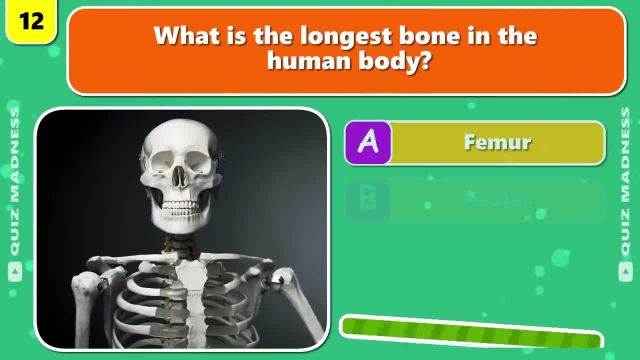 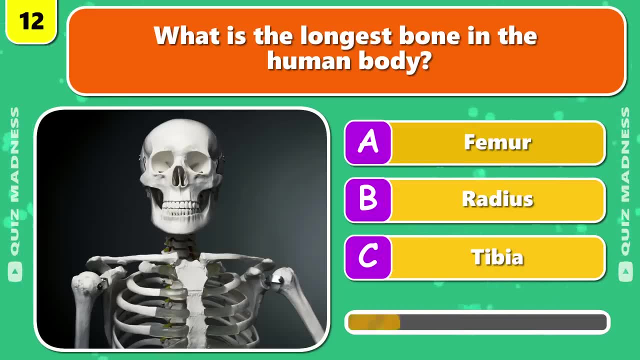 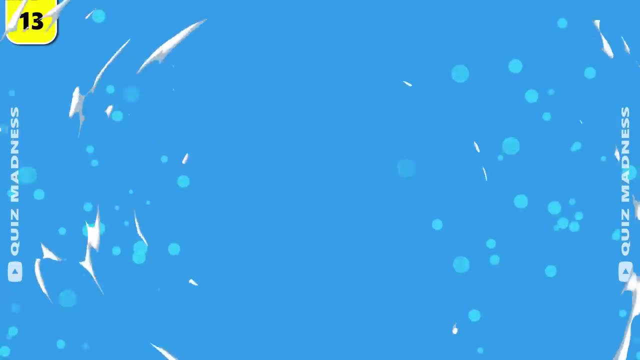 Question 12.. What is the longest bone in the human body? A- Femur, B- Radius or C- Tibia? The correct answer is A- Femur. Question 13. What is the capital city of the United States? The answer is A- The capital city of the United States. 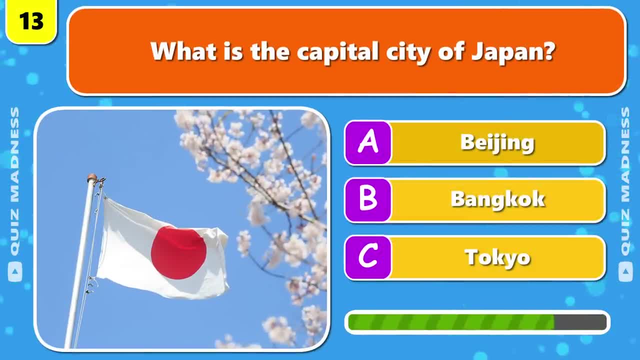 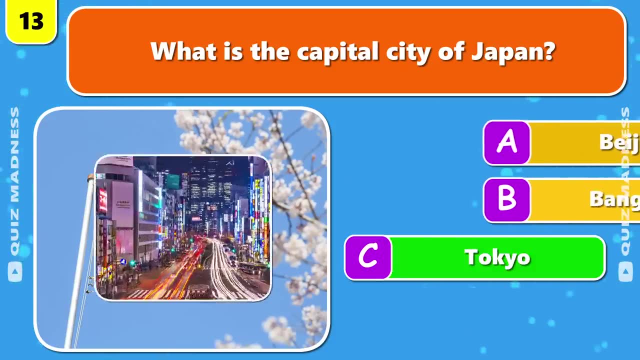 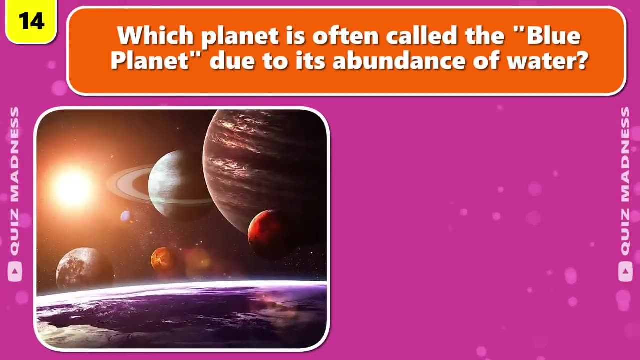 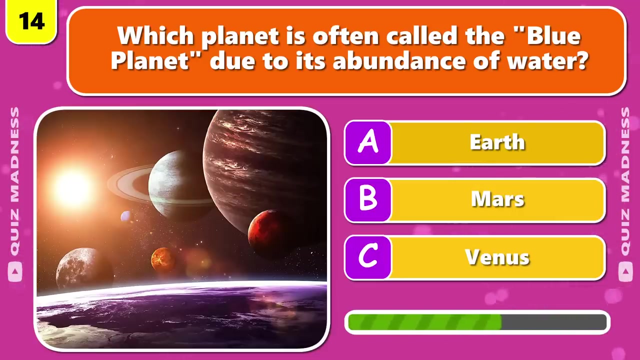 The answer is A- The capital city of Japan. Is it A- Beijing, B- Bangkok or C- Tokyo? The correct answer is C- Tokyo. Question 14. Which planet is often called the Blue Planet due to its abundance of water? A Earth, B- Mars. 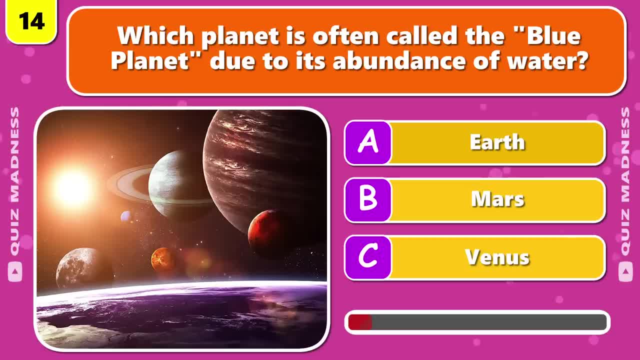 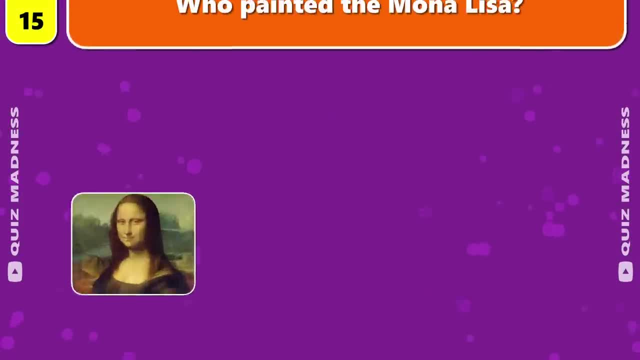 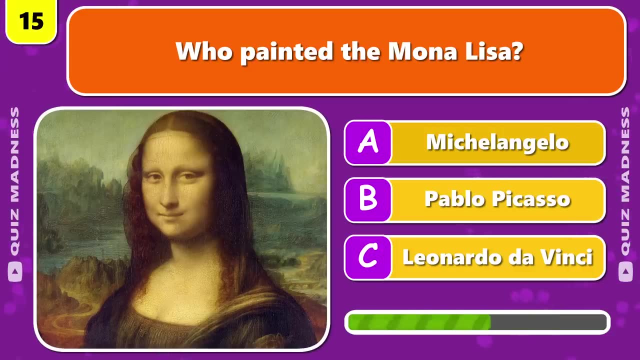 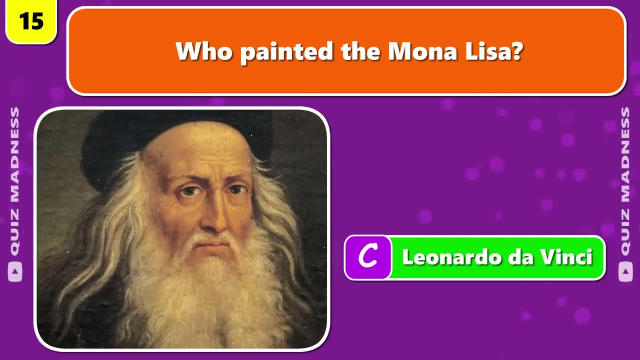 The correct answer is C Earth. The correct answer is C Earth. Question 15. Who painted the Mona Lisa? Was it A Michelangelo, B Pablo Picasso or C Leonardo da Vinci? The answer is C Leonardo da Vinci. Question 16. Which is the longest river in the world? 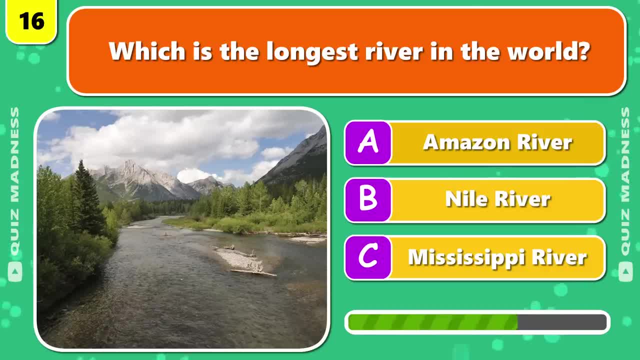 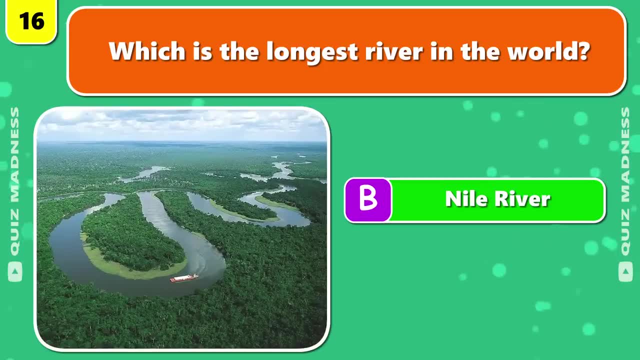 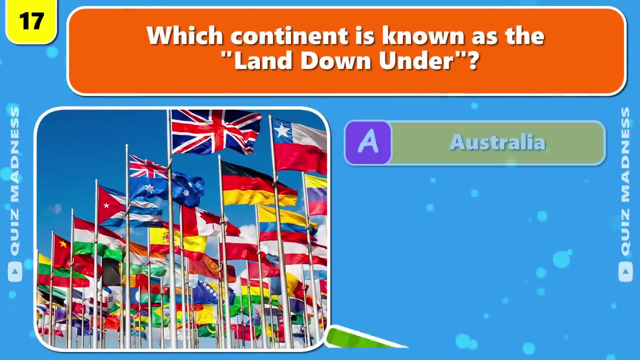 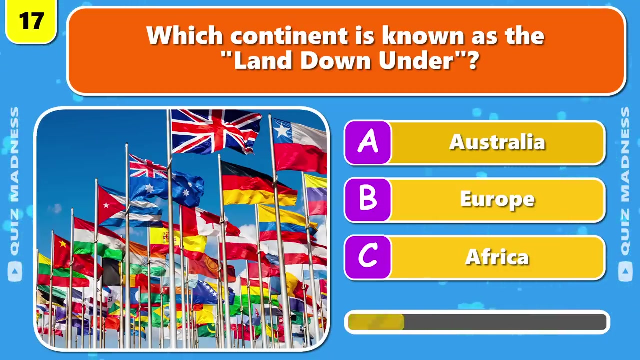 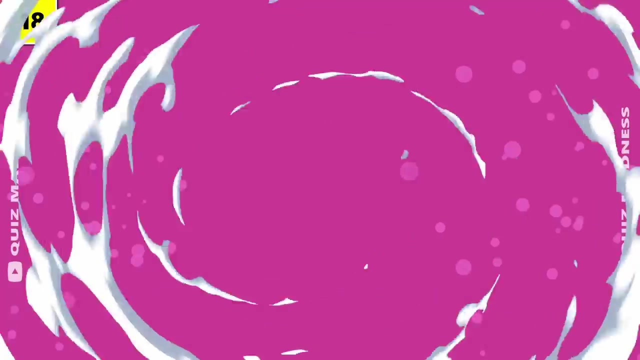 A Amazon River, B Nile River Or C- Mississippi River. The answer is B- Nile River, Question 17.. Which continent is known as the Land Down Under? A- Australia, B Europe Or C- Africa? Correct answer is A- Australia, Question 18.. 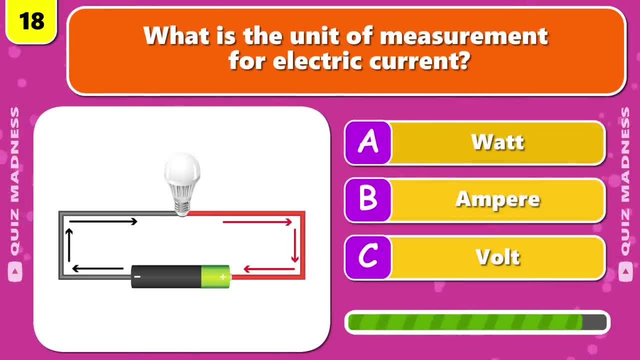 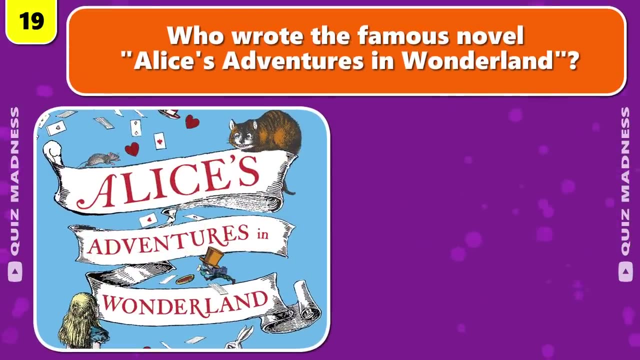 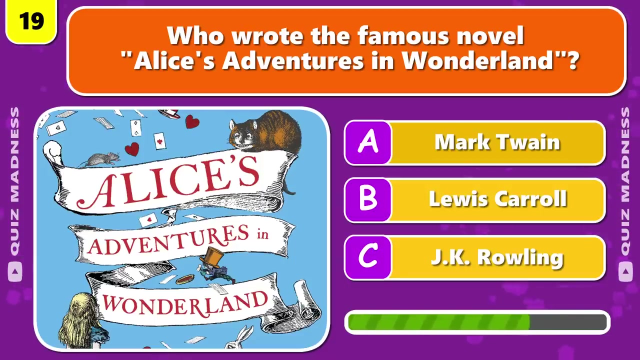 What is the unit of measurement for electric current? A Watt, B Ampere Or C Volt? That would be B Ampere, Question 19.. Who wrote the famous novel Alice's Adventures in Wonderland? A Mark Twain, B Lewis Carroll. 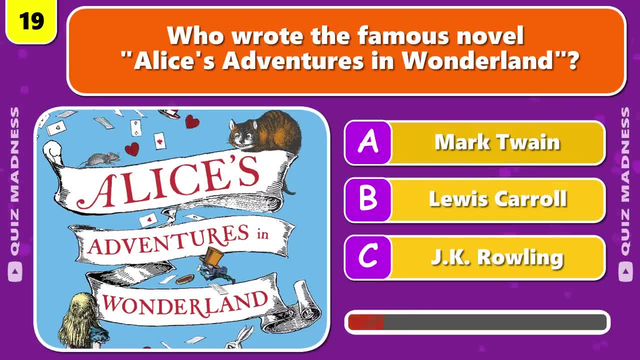 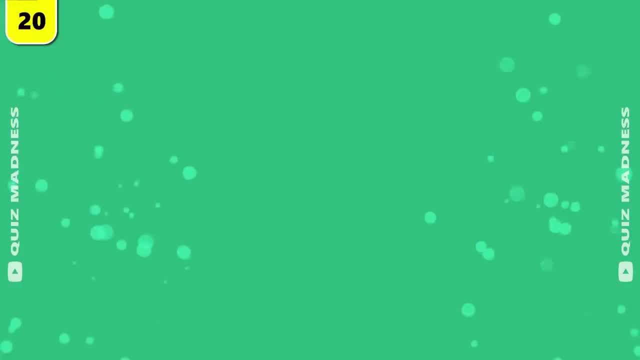 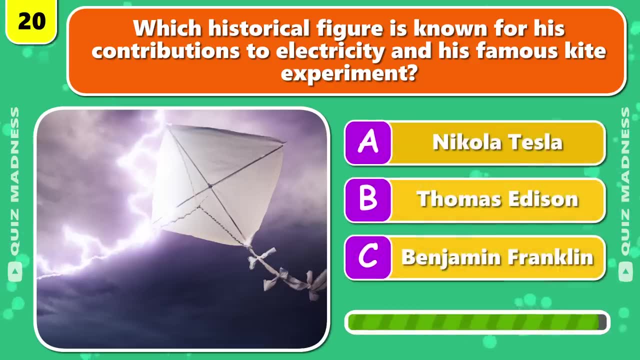 Or C- J K Rowling. Correct answer is A- New York, B- Lewis Carroll wrote it. Question 20.. Which historical figure is known for his contributions to electricity and his famous kite experiment? A- Nikola Tesla, B- Thomas Edison Or C- Benjamin Franklin. 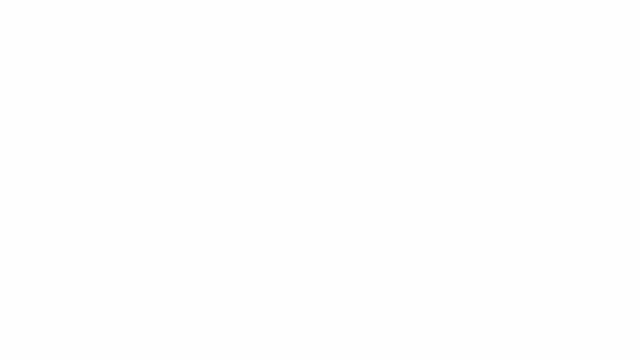 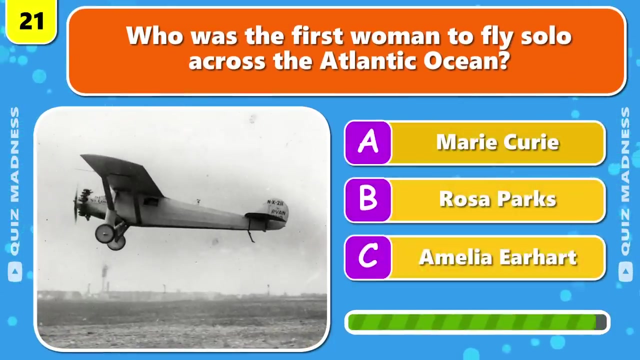 The answer is C Benjamin Franklin, Question 21.. Who was the first woman to fly solo across the Atlantic? A Thomas Edison Or C Benjamin Franklin? Correct answer is C Benjamin Franklin. Who came across the Atlantic Ocean? A Merry Curie. 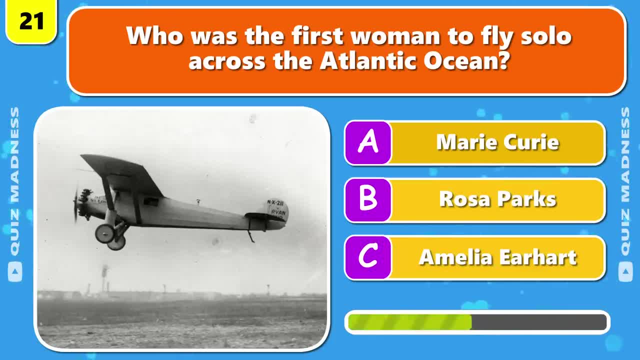 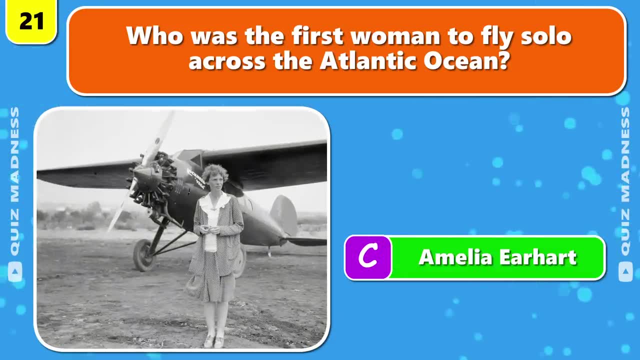 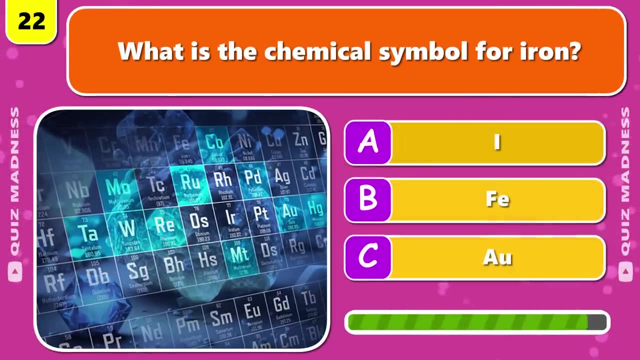 Or C. Tcription B, Rosa Parks, Or C, Amelia Earhart. Correct answer is C, Amelia Earhart. Question 22.. What is the chemical symbol for iron? Is it A, I, B, f, E Or C a U Or C a U? 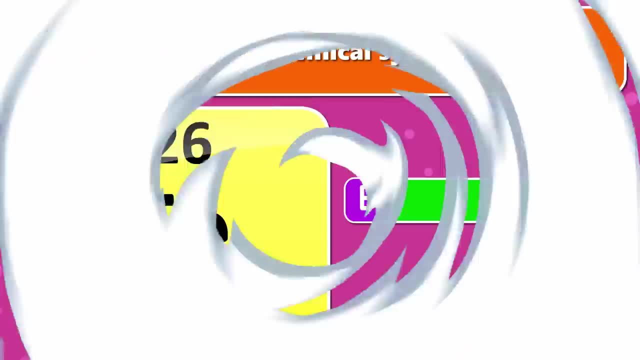 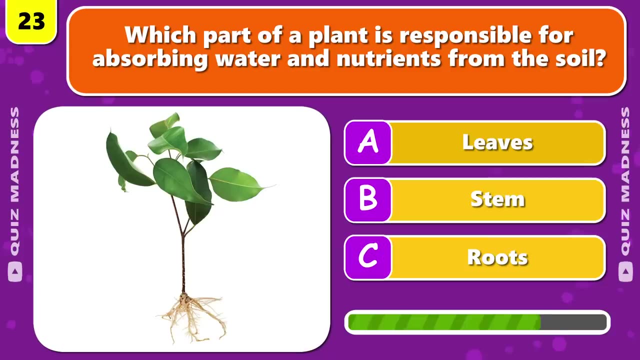 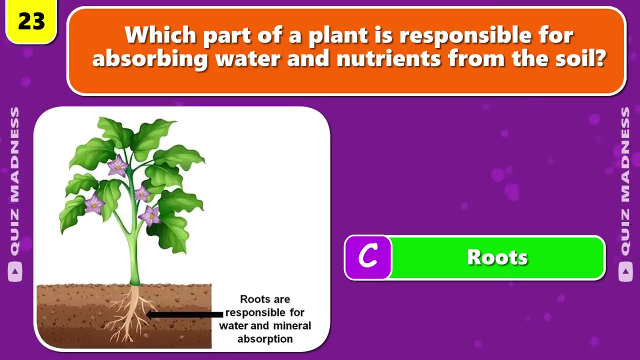 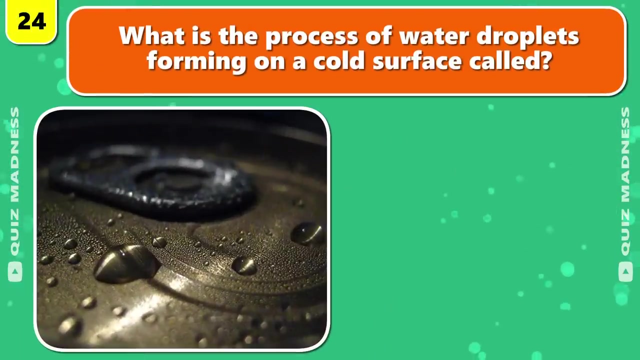 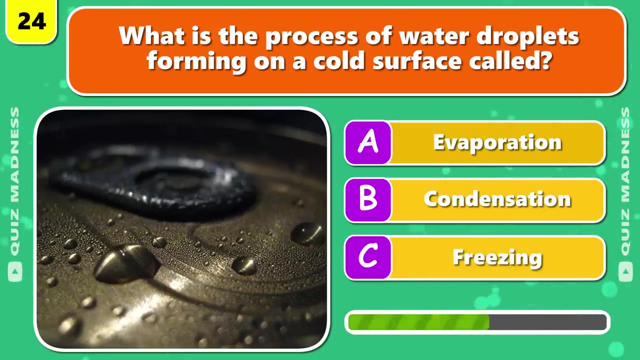 answer is b fe. question 23: which part of a plant is responsible for absorbing water and nutrients from the soil? a leaves, b stem or c roots? yeah, you're right, c roots. question 24: what is the process of water droplets forming on a cold surface called a evaporation, b condensation or c? 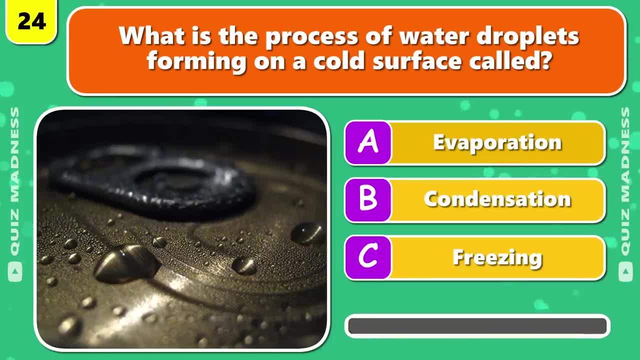 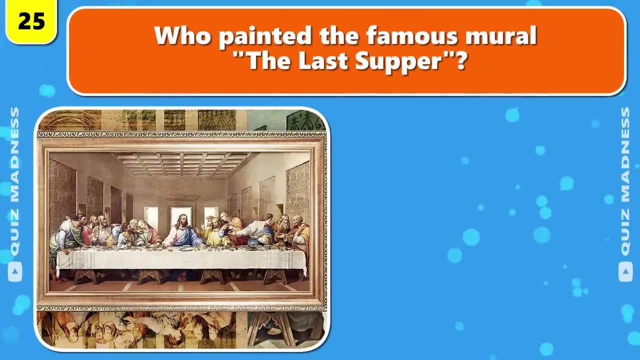 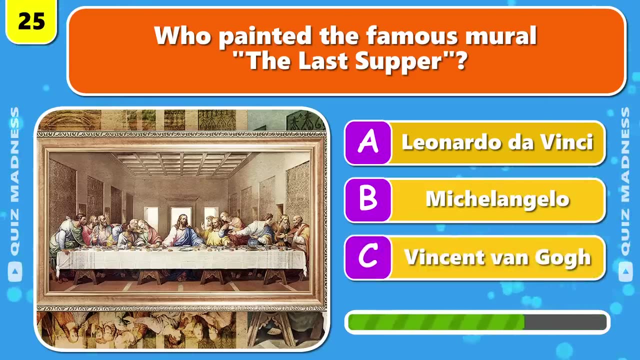 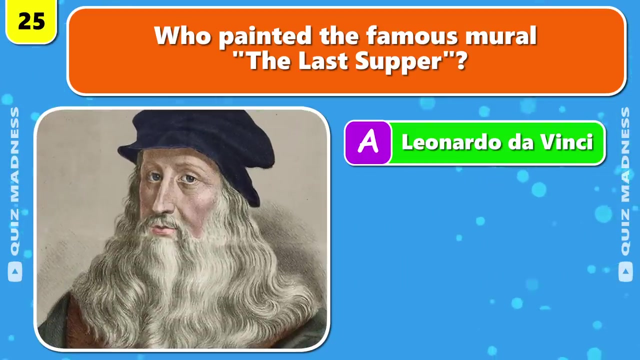 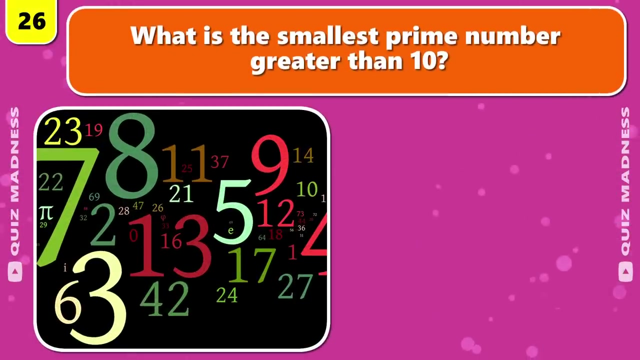 freezing. the answer is b- condensation. question 25: who painted the famous mural, the last supper? a leonardo da vinci, b- michelangelo or c vincent van gogh. that would be a leonardo da vinci. question 26: what is the smallest prime number greater than 10? 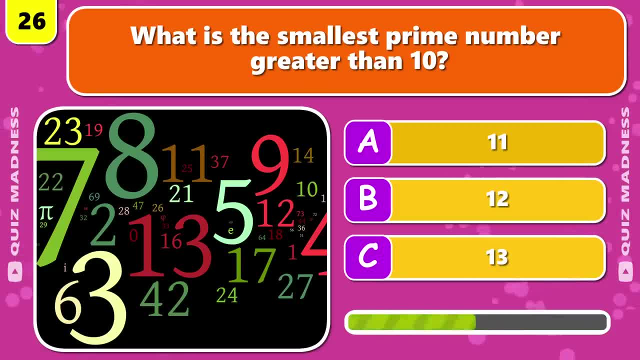 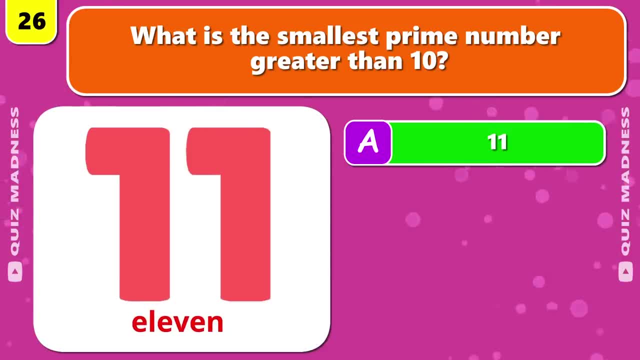 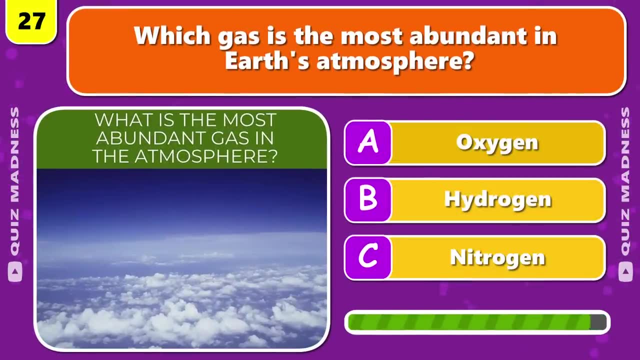 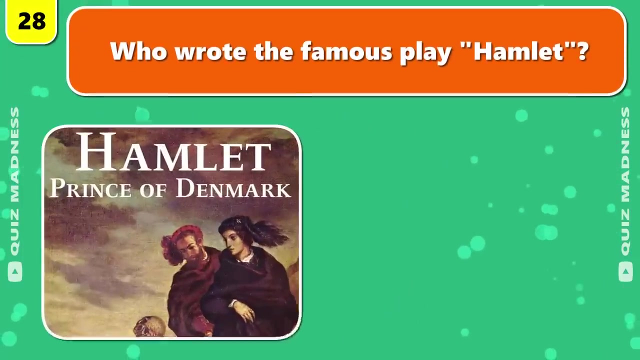 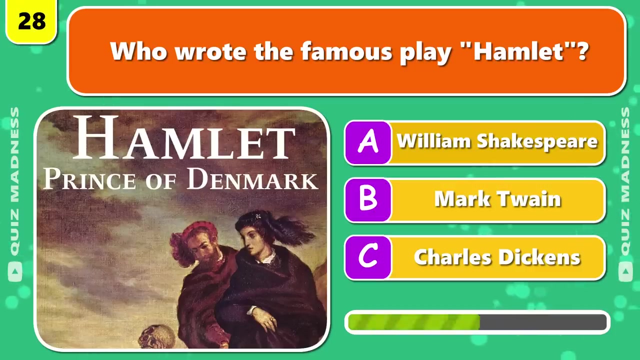 a, 11, b, 12 or c 13.. correct, it's a 11.. question 27: which gas is the most abundant in earth's atmosphere? a oxygen, b hydrogen or c nitrogen? the answer is c nitrogen. question 28: who wrote the famous play hamlet? was it a william shakespeare, b mark twain or c? 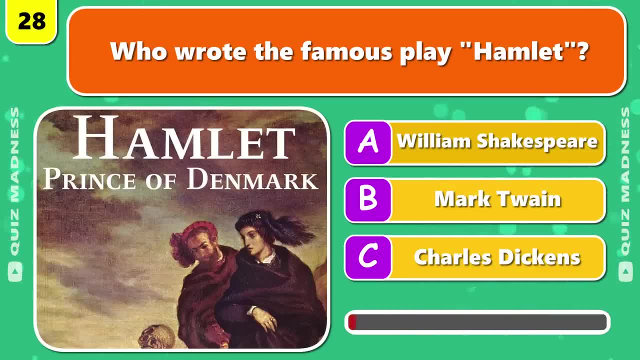 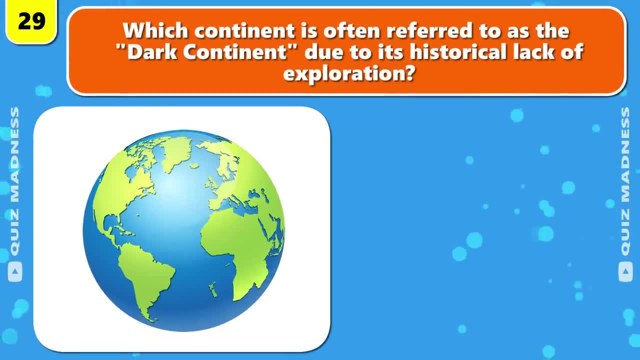 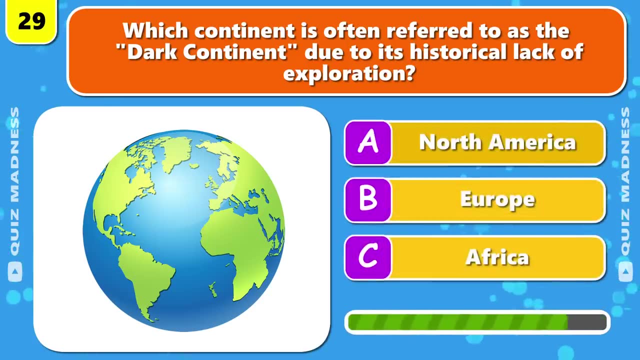 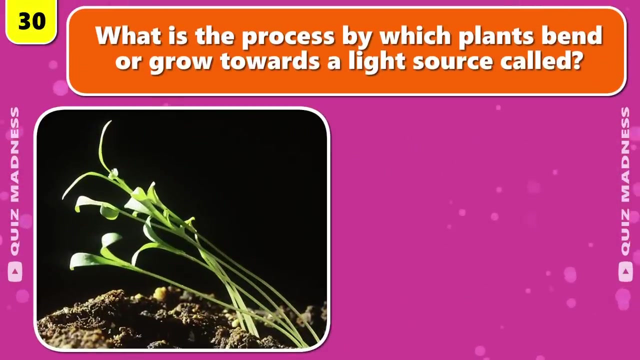 charles dickens. correct answer is a- william shakespeare. correct answer is a logbook. question 29: which continent is often the dark continent due to its historical lack of exploration? a north america, b europe or c- africa? if you said see africa, you are correct. question 30: what is the process by which plants bend or grow?